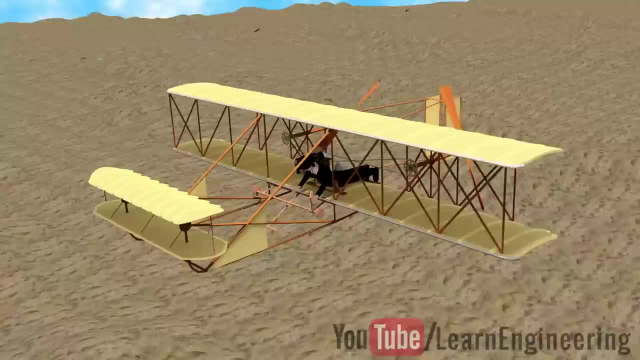 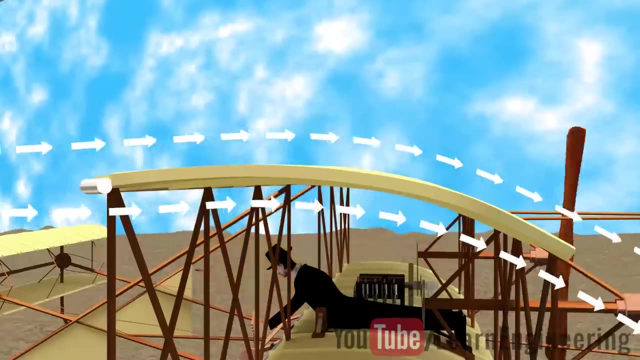 Also made use of this same airfoil principle. Even though their airfoils were a simple curved shape, it was sufficient to produce a good downwash. More specifically, their airplane had two such airfoils. One more idea to increase the lift force. 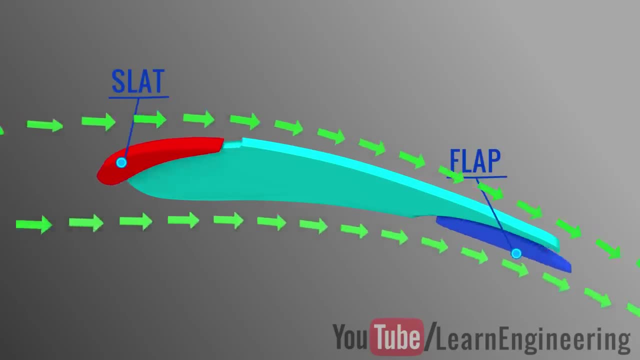 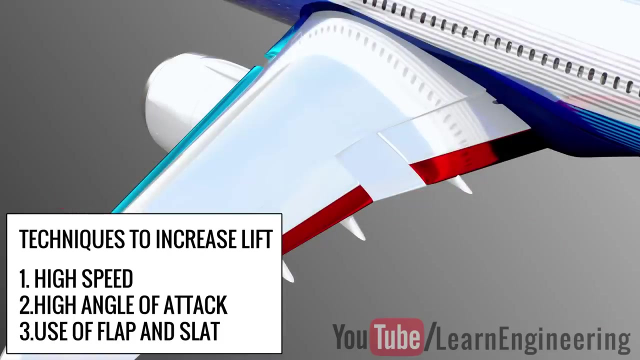 is by altering the airfoil shape. like this, The alteration in shape will definitely increase the downwash and the wing area, hence giving greater lift. In short, there are three techniques to increase the lift of an airfoil. Let's apply this airfoil knowledge to the airplane. 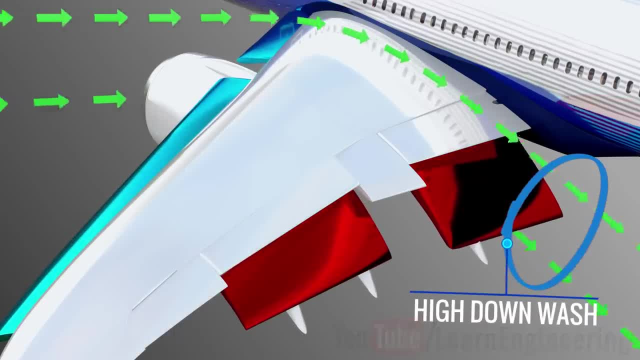 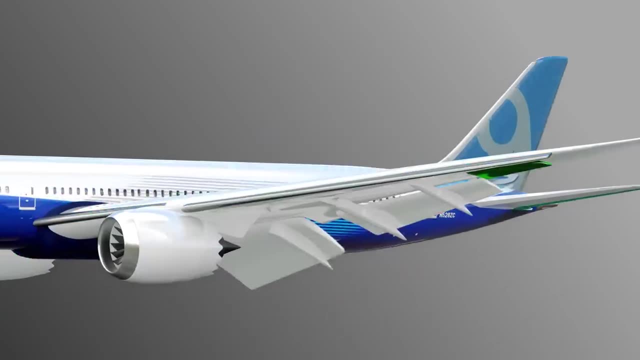 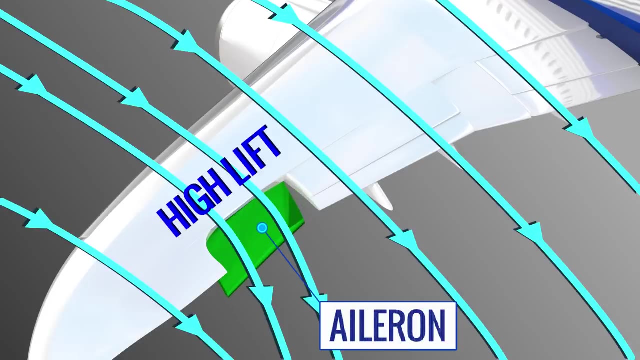 If we activate the flaps and slats, it increases the downwash and increases the lift. The ailerons can move up and down and for that reason the lift force can decrease and increase respectively. To do this we need to set a different angle for the foot Airsoil. Here are two different angles to alter the lift force. At the tail of the airplane you see a compact airfoil and both wolf snake are agreeable. As in the Episode I, there is no difference between the active weight and lift, but the lift Doing it from the tail of the airplane is less likely. 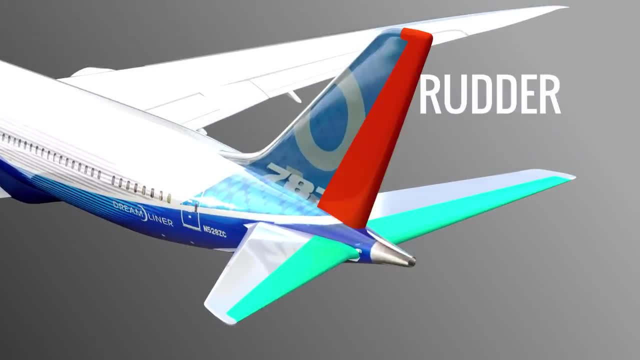 the lift force can be the entire aircraft. fuss the lift of the tail of the airplane and increase the lift. you can see two attachments: the rudder and the elevators. By adjusting the elevators you can control the vertical force on the tail. 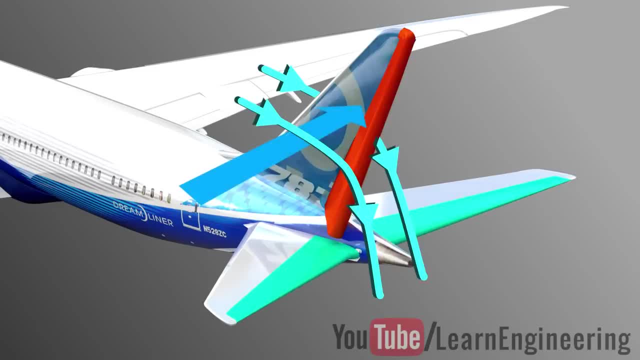 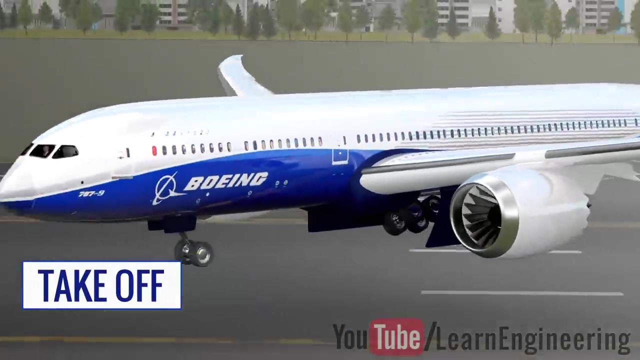 By adjusting the rudder, you can control the horizontal force. Now let's get into the most interesting part of the video: controlling the aircraft using these simple wing attachments. Let's start with the take-off part of the flight: To get the airplane to take off from the ground. 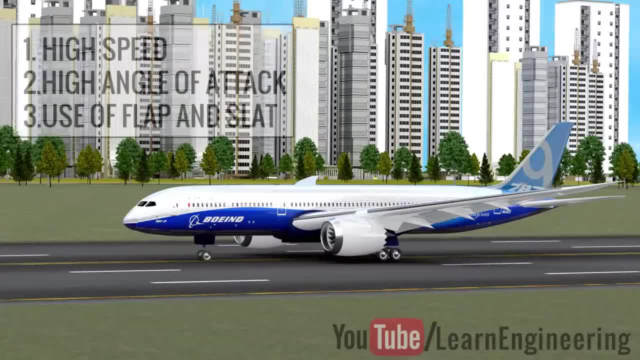 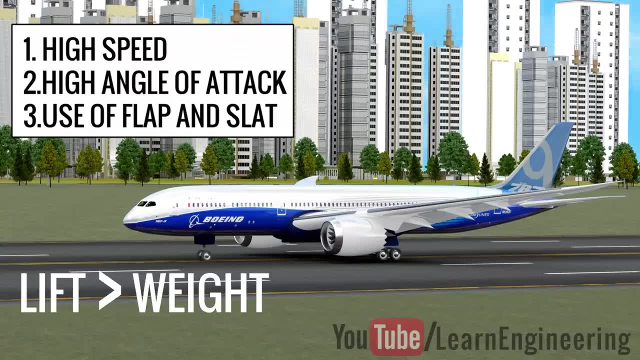 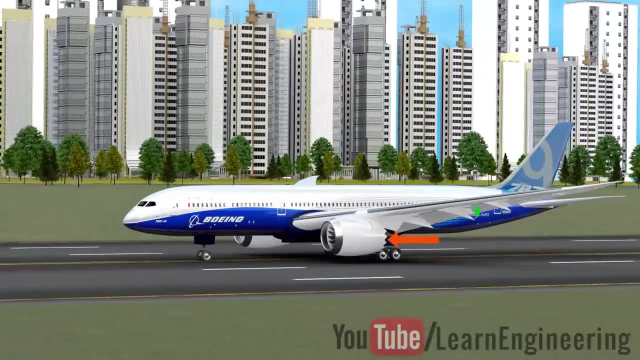 what you have to do is increase the lift force using various techniques and make sure that this force is more than the gravitational pull. Pilots apply all of the three lift increase techniques together for a successful take-off. First, the speed of the airplane is increased by increasing the thrust of the engines. 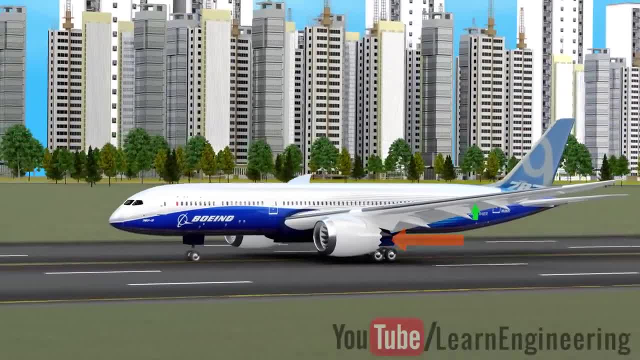 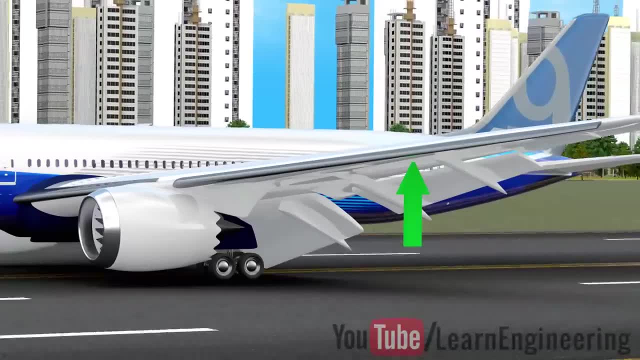 When the airplane's speed is high enough, the pilots activate the flaps and slats. Lift is further increased due to this. When the airplane is ready for take-off, they activate the flaps and slats. They activate the elevators upwards. 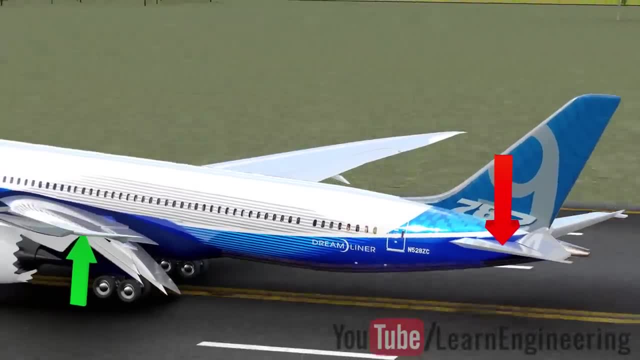 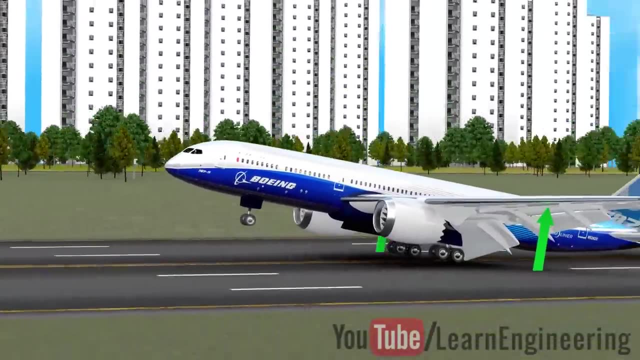 The tail force tilts the airplane as shown and the angle of attack of the airfoil will be increased. The lift is suddenly increased due to this and the airplane takes off. Usually, an angle of attack of 15 degrees is maintained for the take-off. 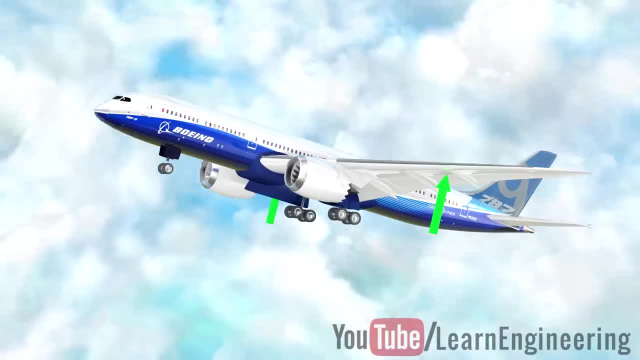 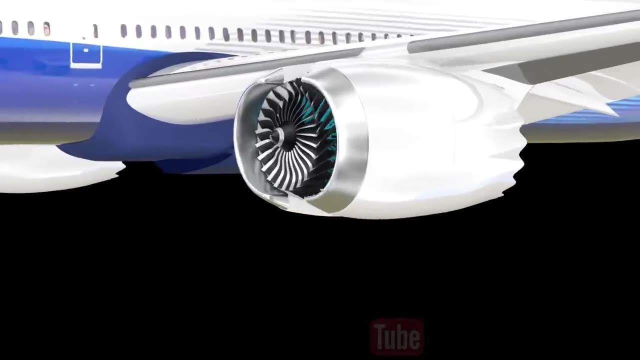 In all these discussions we are talking about the engine's thrust. But how is the engine able to generate thrust? Modern airplanes use special kinds of engines called turbofan engines for this purpose. In this, the fan's reaction and the reaction force of the exhaust. 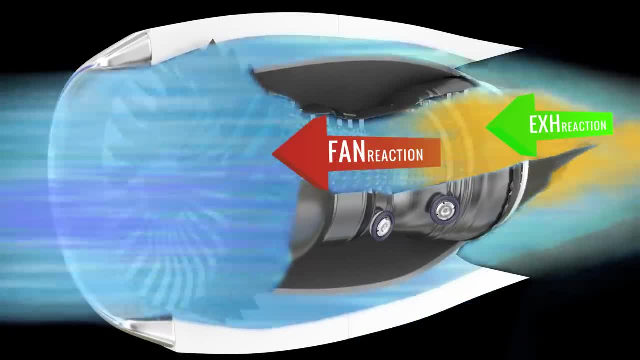 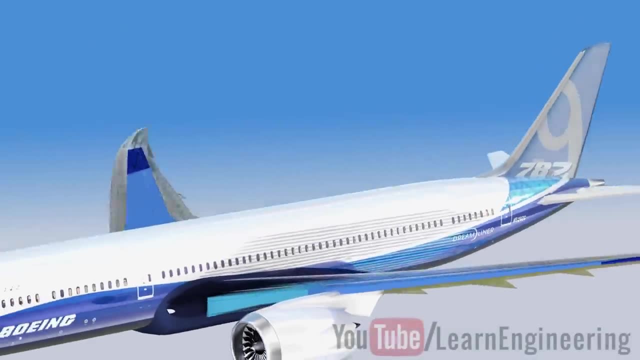 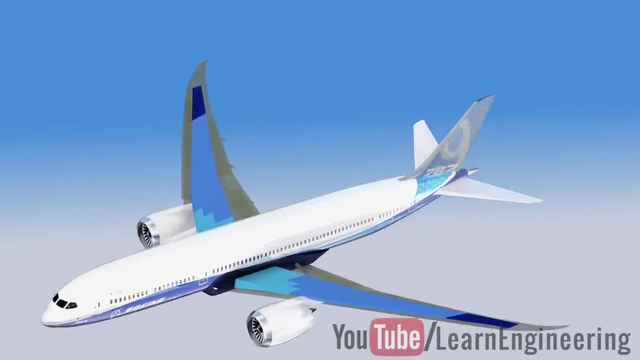 give the necessary thrust force. By burning more fuel, the pilot can achieve more thrust. The fuel of an airplane is stored inside the wings After the take-off. next comes the climb phase of the aircraft, As long as the engine's thrust is more than the drag. 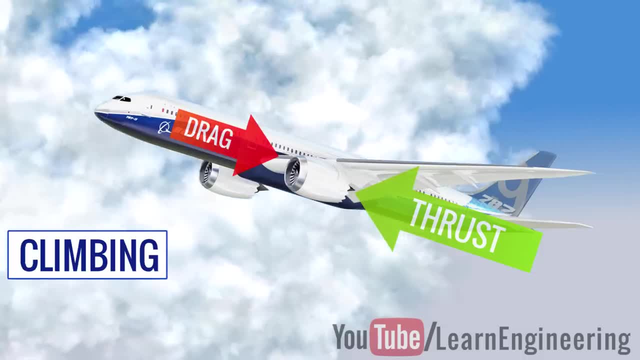 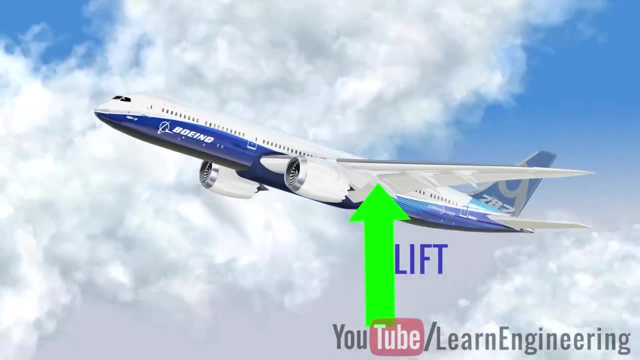 the speed of the airplane will keep on increasing. The greater the speed, the higher will be the lift force. This will cause the airplane to go up. When the airplane reaches level flight, there won't be any acceleration or change in altitude. You can see that with this condition, 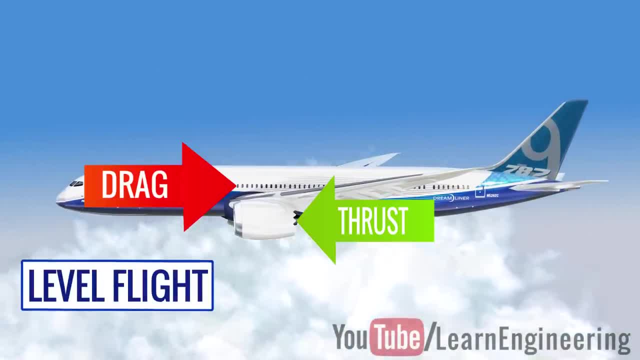 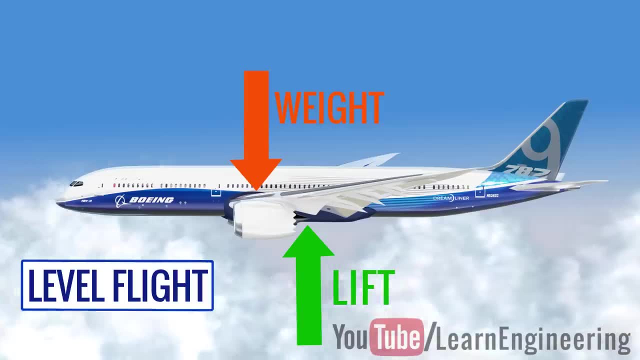 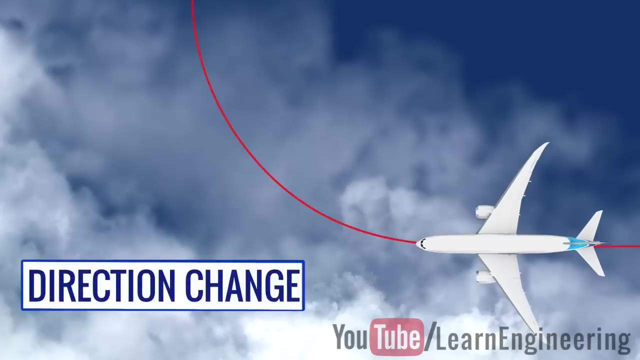 The thrust should be exactly equal to the drag and the lift should be exactly equal to the weight of the airplane. Now let's discuss the most crucial part: How does an airplane move? How does an airplane change direction? You might think that just by adjusting the rudder. 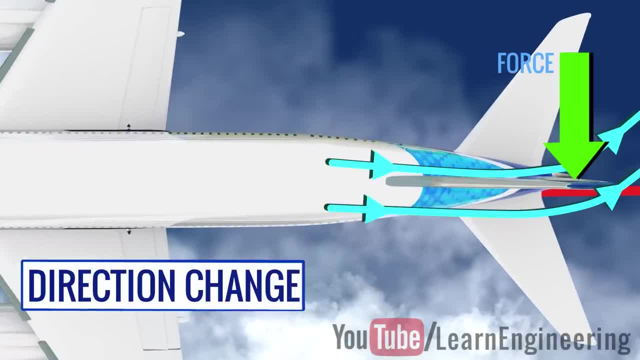 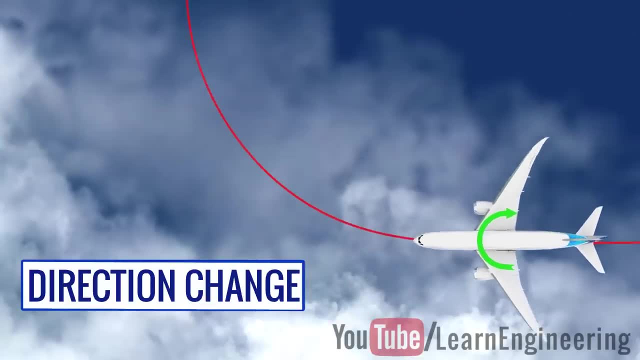 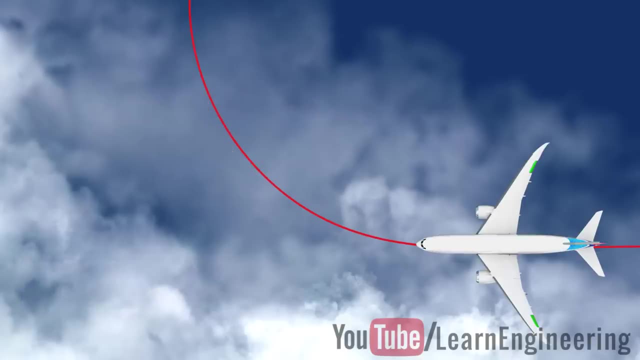 you would be able to do this. The rudder produces a horizontal force and this force can turn the airplane. However, such a direct change in direction will cause discomfort to passengers and it is not a practical method To make a turn, as shown. 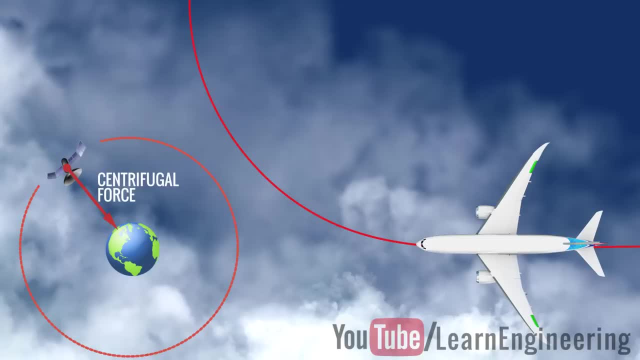 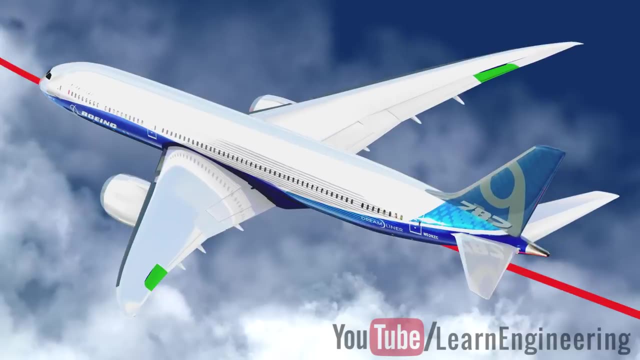 what you need is a centrifugal force. Let's see how pilots achieve this centrifugal force. Pilots just make one aileron go up and the other aileron go down. The difference in the lift force will make the airplane roll. 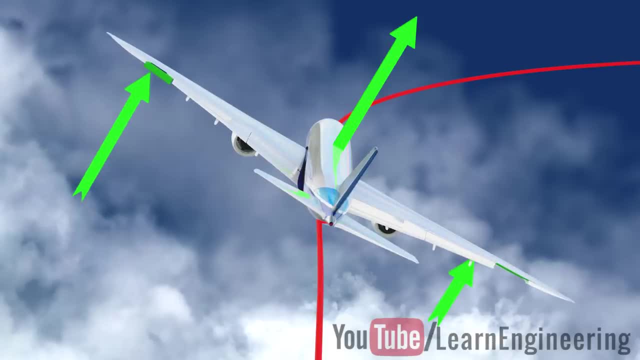 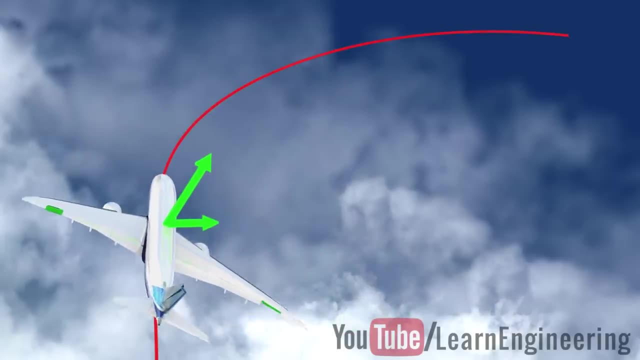 In this roll condition the lift is not vertical. The horizontal component of the lift can provide the necessary centrifugal force to bank the aircraft. This way, the pilot can make a turn of any radius, depending upon the angle of roll and the speed of the airplane.